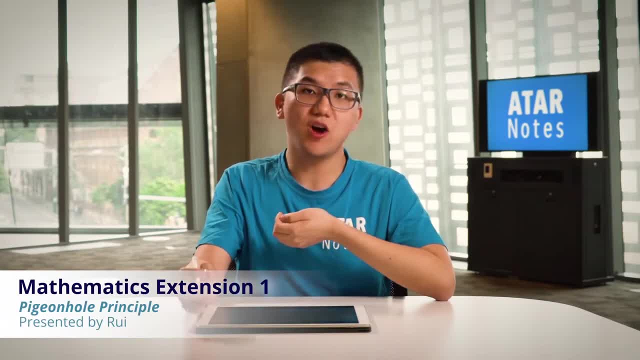 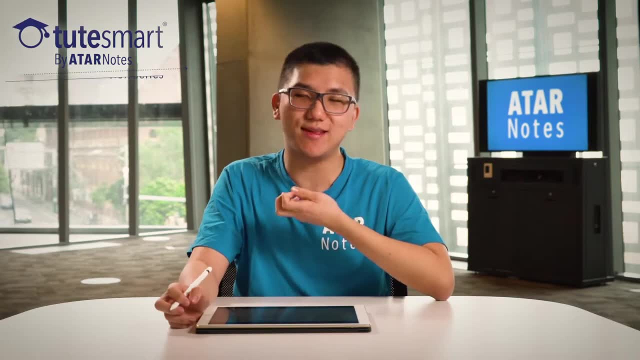 So today I want to talk about a year 11 concept and that is the concept of the generalized pigeonhole principle and, loosely speaking, I'm pretty sure most of you guys have figured this out already, but, yes, it pretty much is common sense. So the principle states that if you have, say, n pigeons, 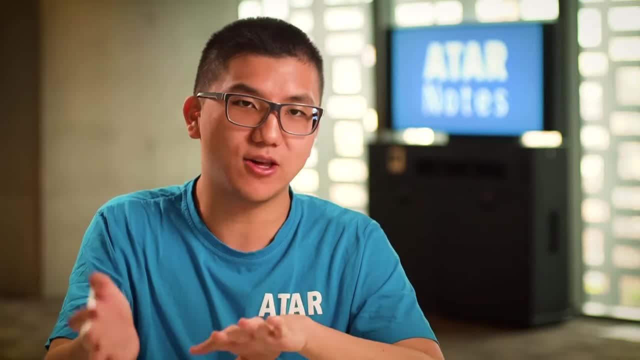 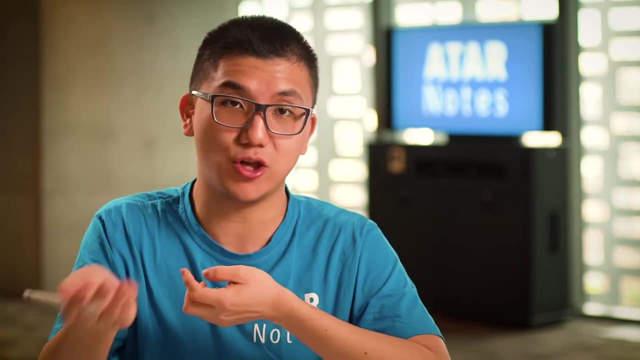 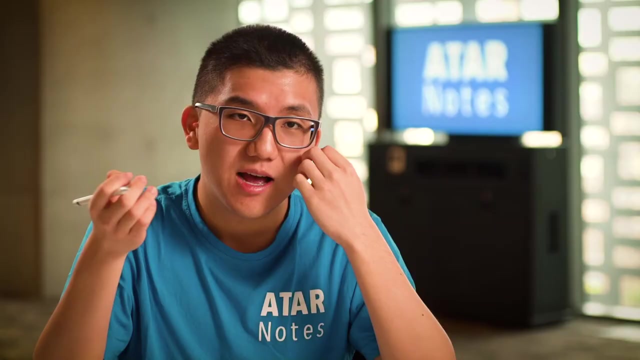 and then you're given k pigeon holes to just dump all of the pigeons in. then it just turns out that at least one of the pigeon holes must contain n divided by k pigeons, and that's fairly intuitive enough to understand in terms. I can just do some very nice maths with it somehow, but I found that 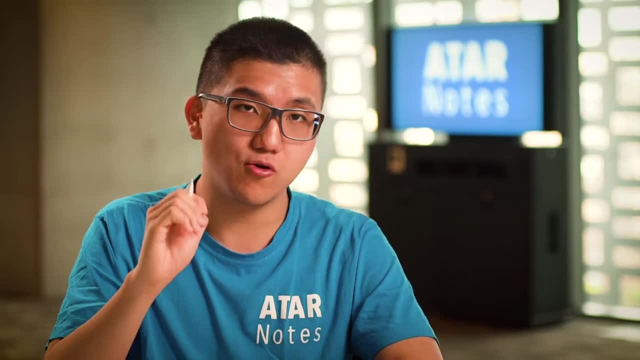 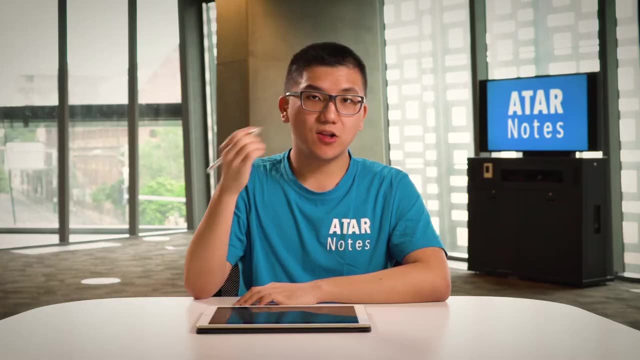 when I first started getting into these problems, the hardest thing for me to do was figure out: one, what are the pigeons? and two, what are the pigeon holes? Loosely speaking, I like to think of things this way: I like to treat the pigeons as some object of interest and I want to treat the 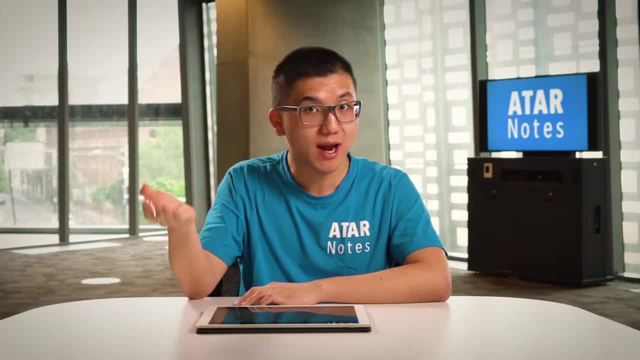 pigeon holes as some favourable characteristic or trait of the pigeons. So I'll go through my questions and then I'm going to go through the questions and then I'm going to go through my questions and then I'm going to go through my questions and then I'm going to go through my. 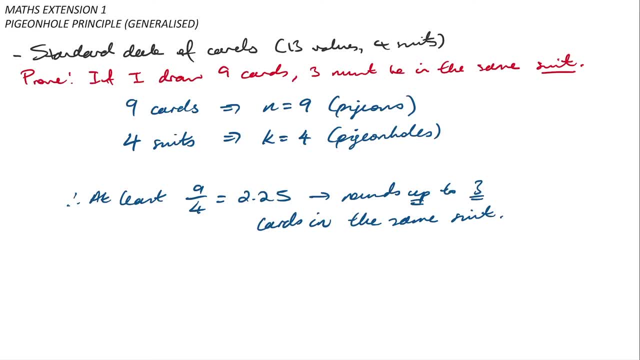 example again. You'll see here that I have a standard deck of cards and, for those of you don't know, there are 52 cards in the decks involving 13 values and four different suits. and I'm just going to do a very simplistic example where I say: oh, if I draw nine cards, then three. 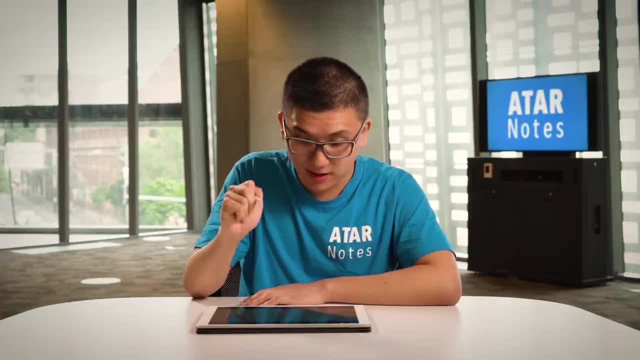 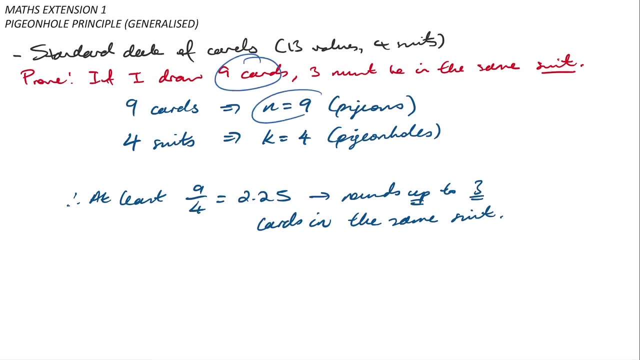 must be in the same suit. Notice how I've actually given away the object and the characteristics straight away. I've given it away that I'm interested in nine cards, so I'm taking n equals nine pigeons. and because I'm interested in the suits, and I know that there's going to be four suits, I'm going to 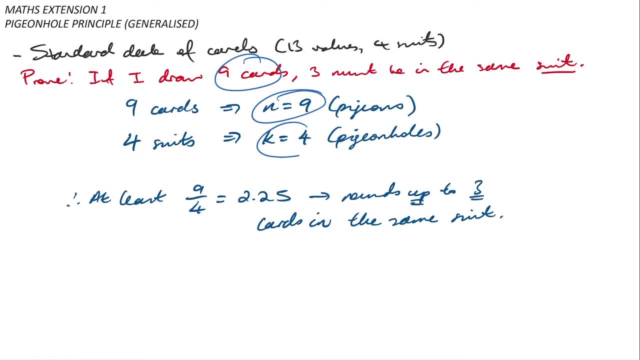 take k is equal to four pigeon holes, and then pretty much I just literally use my theorem or principle So I'll say: well, okay, at least nine divided by four, which is equal to 2.25 cards are in the same suit, but the good thing about the pigeon hole principle is that I can always round. 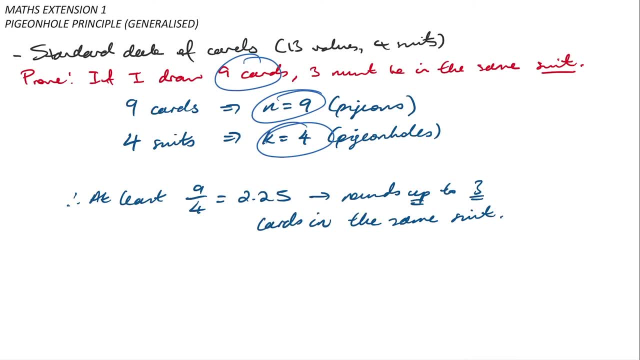 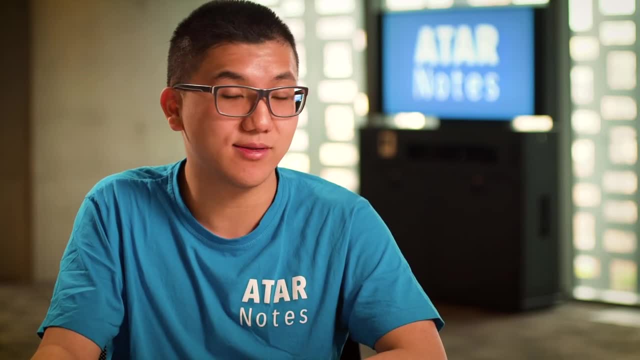 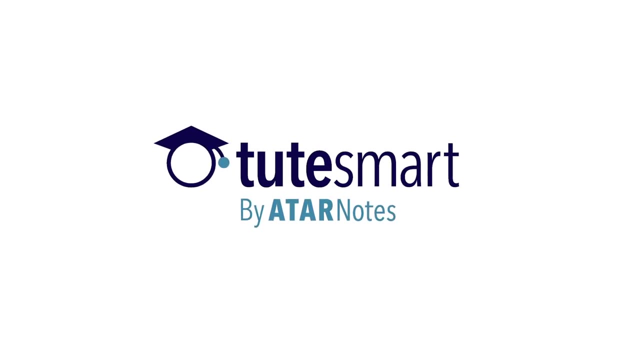 it up to saying. in fact, there will always be at least one pigeon hole. with three cards in the same suit, Very simplistic application, but there's not really that much else to it. Thanks everyone. I'm going to end the video here. I hope you enjoyed it and I'll see you in the next video.